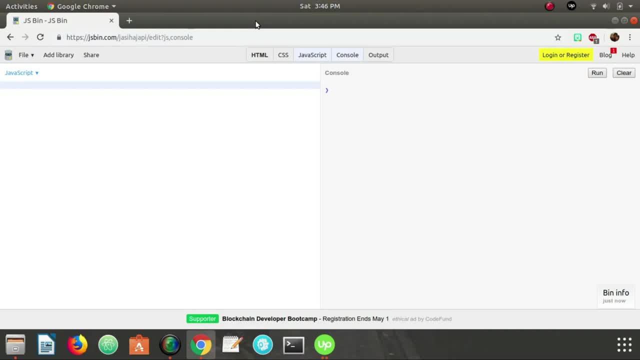 is a building where things are manufactured. So in the programming sense a factory is just an object that creates or manufactures different objects. So why is this useful? Why do I need an object to create my objects? Why don't I just create them on the fly when 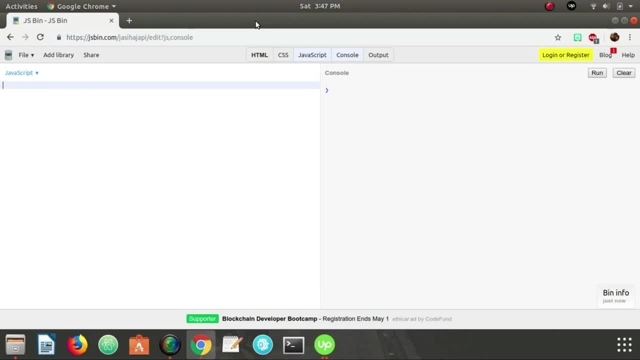 I need them. using the new keyword Well factories allow you to handle all of your objects So you don't have to worry about all of your object creation in a centralized location. So you don't have to worry about having all kinds of constant. object equals new object. 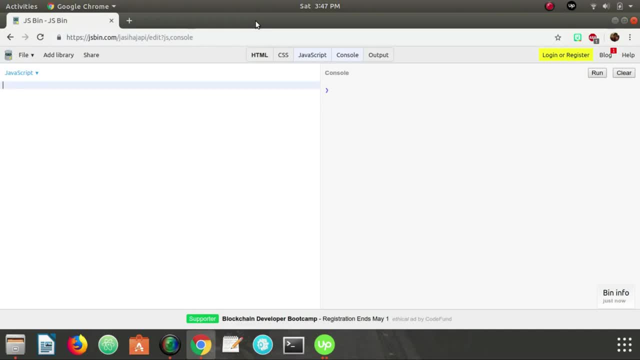 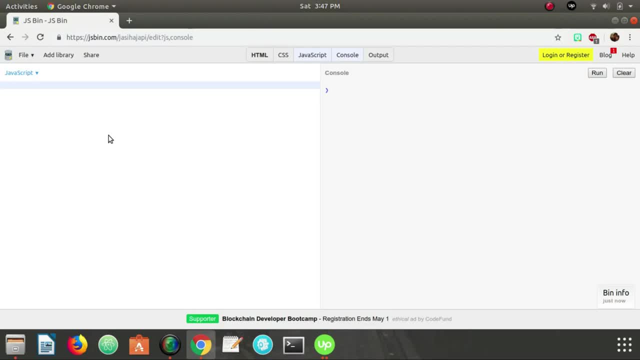 look at the code. So we're going to set up a scenario. So let's say I own a software business and I have employees. I have two types of employees. I have my developers who write code for new features, and then I have my testers who write tests to make sure those 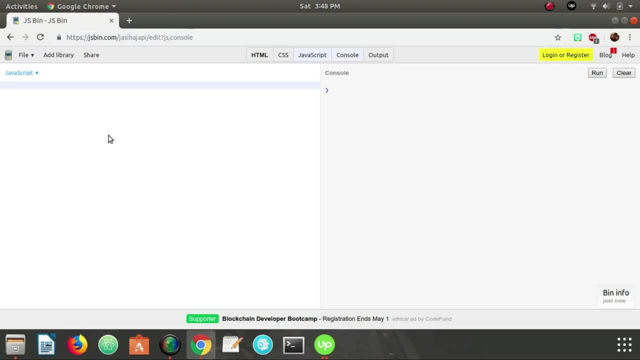 features are working And I want to set up a database so I can keep track of all my employees. So let's go ahead and create our developer object constructor, And a developer is going to have a name, so we need to take in a name, And so we're going to say this dot name equals. 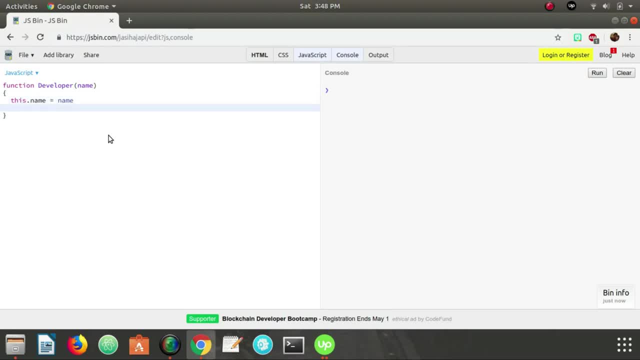 name And we also want to be able to tell what kind of employee this is. So let's say, this dot type equals developer, Now we can create our tester. Likewise, it's going to have a name. This dot name equals name and this dot type equals tester, And now we can create our factory. 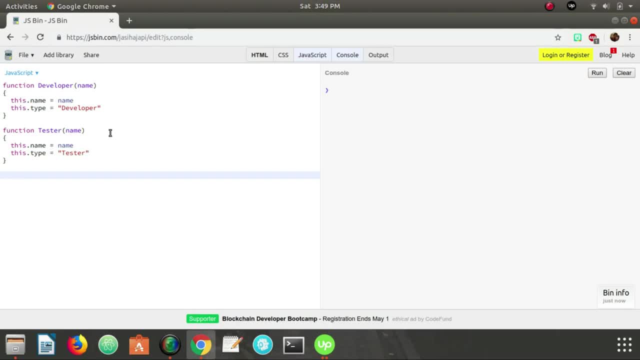 our employee factory. um, so let's say, function, employee factory and factories in the the. the, in the most base case, is going to at least have a create method, and this is going to be responsible for actually creating your different objects that you need, and create is going to take in in this case it's going to 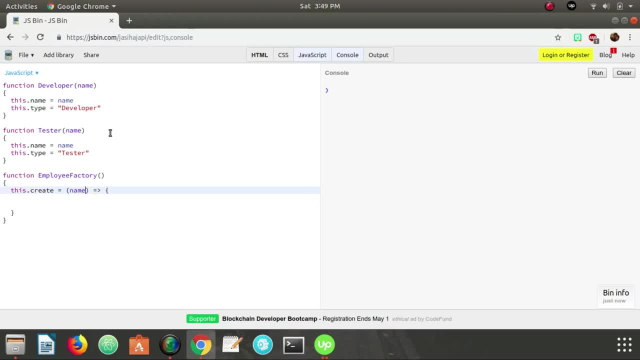 take in a name for whatever type of employee you want to create, whether it be a developer or tester, and then it's also going to take in the type, so it knows which one to create. so let's say, our type is just going to be an integer, and type 1 employees are going to be developers, while type 2 employees 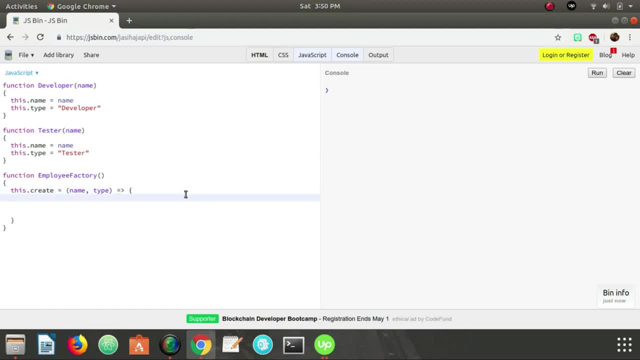 are going to be testers, so we need to actually get a switch going based off of the type, so we can know which one is going to create, which one is going to create, which one is going to create what type of employee you want we want to create. so, in the case it's one, we want to return a new. 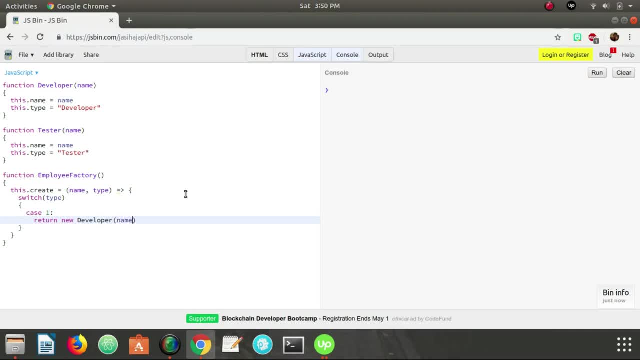 developer with the name that we passed in. name break and case type is two. we want to return a new tester with the type with the name of name and break, and that's pretty much it for our factory class. we can actually get to using it now. so let us say: 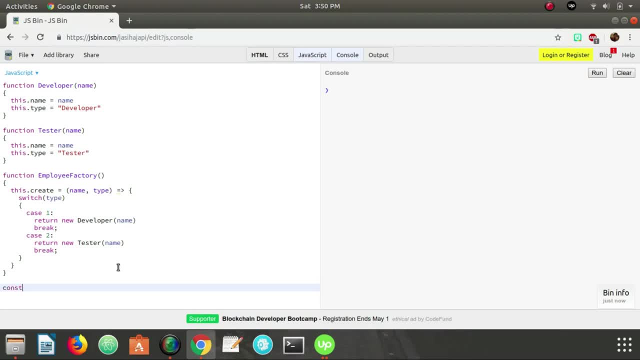 we have our, let's create a new instance of our factory so we can say const employee factory equals new employee factory factory. and now let's actually, let's get our database going. like I said, we, our database is just going to be an array, so we can just create an array of employees is equals to empty array. and let's. 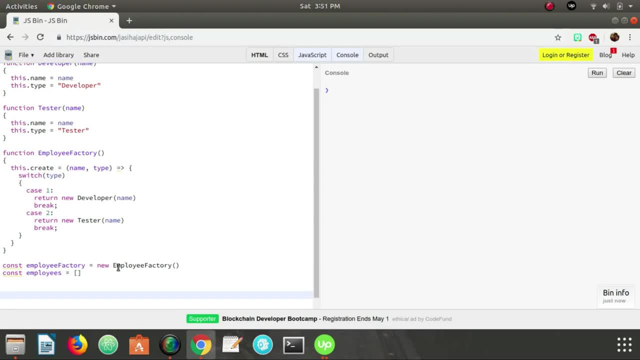 start inserting employees into our employees array so we can say employees dot push, employee factory dot create. and this create is going up here, takes in a name of our new employee and the type of the employee you want to create. so let's say we want to create a new developer. 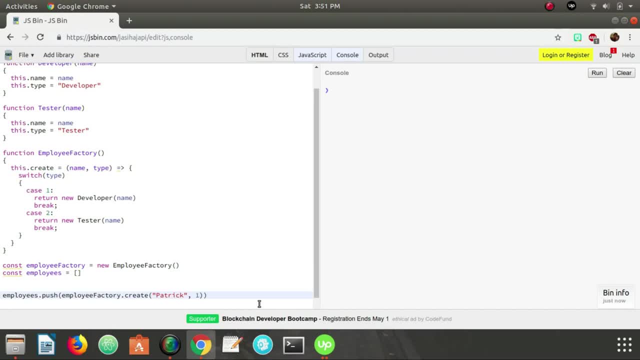 named Patrick. so type one Patrick and there we go. so let's actually get some some away to to kind of verify that this is working. so we're going to, let's, we're going to create a function, say, which is actually going to print out the information of whatever employee we want to create our an employee. 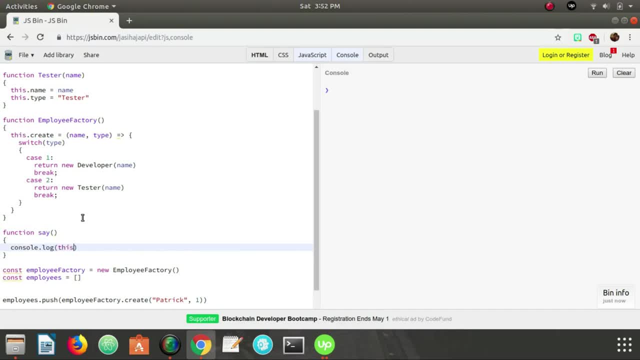 want. so we can say: console dot, log this dot. well, let's say, hi, I am this dot name and I am a this dot type. and then we can say let's loop through all of our employees and call, say, with each of the employees. in this case we only have one. 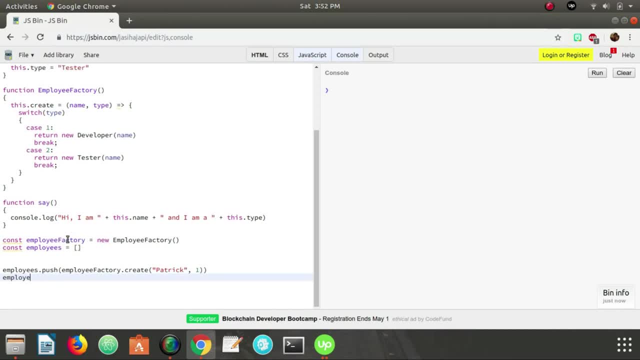 employee, so let's add another one before we do that. so let's say we want to add a tester, we can say: employee factory dot, create a tester named John, so type to name John. so now we're going to loop through employees with a for each loop. 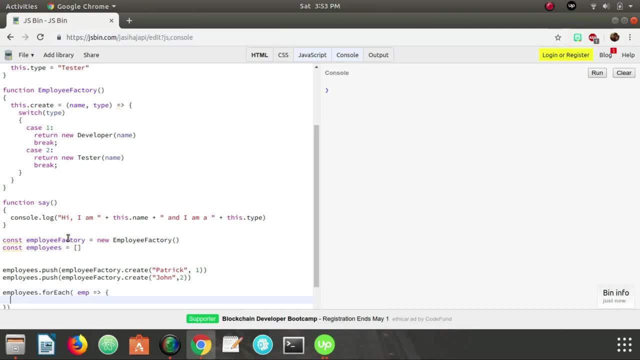 for each employee we want to call say on it. so say dot call and pass in the employee to be the this reference for whatever employee that is. so I have two employees, Patrick and John. I'm going to call say for each of these employees using that employee. 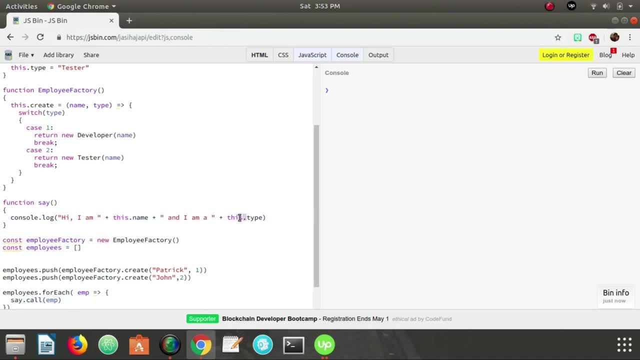 as the this reference for that call. so let's go ahead and let's run it to see what it does. say: hi, I am Patrick and I am a developer. hi, I am John, I am a tester. that's perfect. that's exactly what we're looking for, and we can add more employees here if we want, we can. 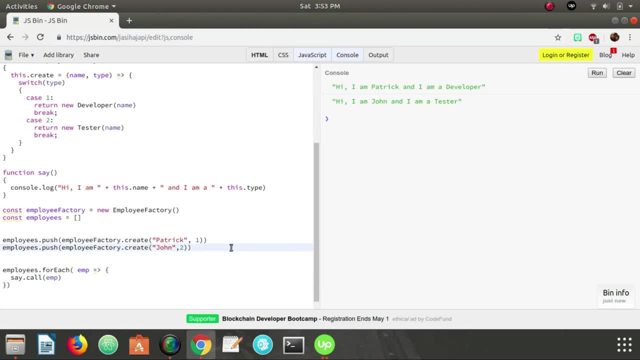 say we can add as many employees as we need. so let's say we want to add some more developers, or developers. let's call this person Taylor, Jamie. we can get another tester in there. let's name him Tim and we can rerun it. hi, I'm Patrick, I'm a developer, John Taylor, developer tester, or Jamie.